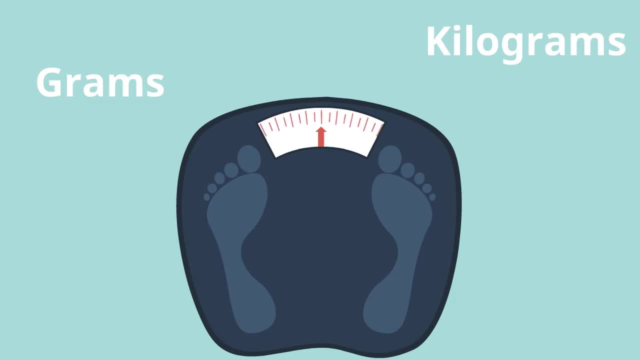 We use grams if we are measuring things that are light and we use kilograms if we are measuring things that are heavy. There is a short way of writing grams and kilograms, Just like there was a short way of writing metres by writing m, and kilometres by writing km. 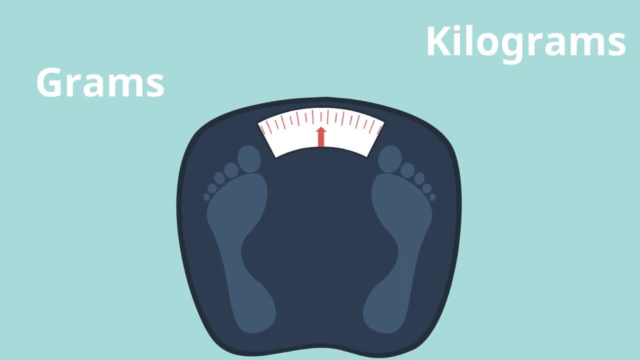 Can you pause the video and write down what the short way of writing grams and kilograms are? Pause the video and give it a try. Well, the short way to write grams is by writing g and the short way of writing kilograms is kg. 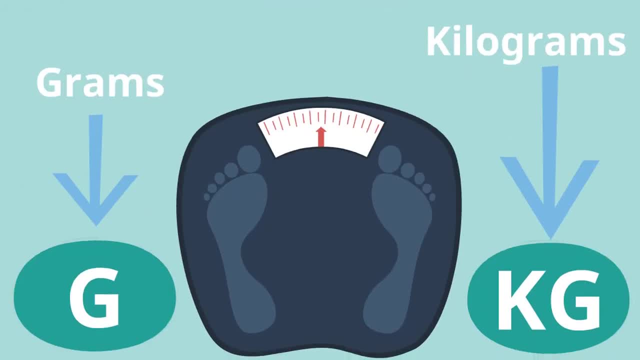 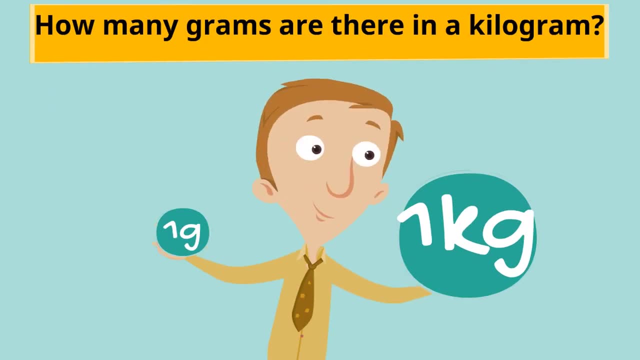 Remember we said we use grams for lighter objects and kilograms for heavier. Well, how many grams do you think there are in one kilogram? If you're very sharp, you might notice that little word kilo before the word gram in our bigger unit. 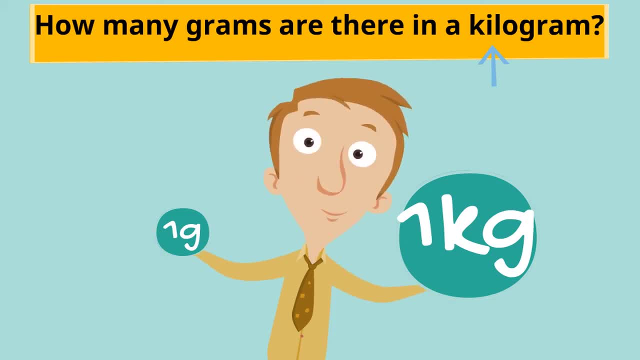 And if you can remember from last week's lessons on length, we saw that word kilo there as well. So if you're very sharp you might notice that little word kilo there as well. So that might help you figure it out. 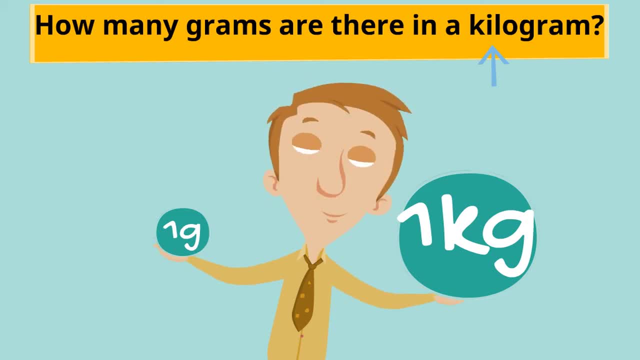 Pause the video and write down how many grams there are in a kilogram. Well, did you get it right? There are 1,000 grams in a kilogram. Remember that word kilo means 1,000 of, just like a kilometre. 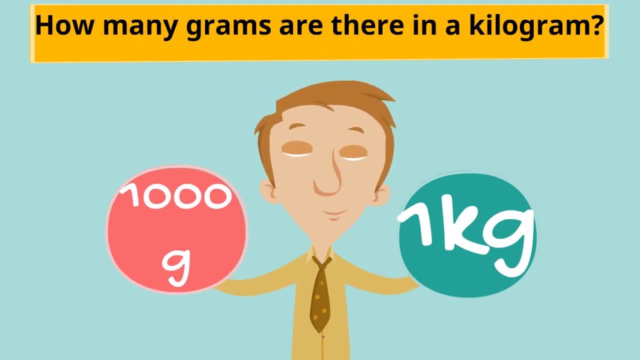 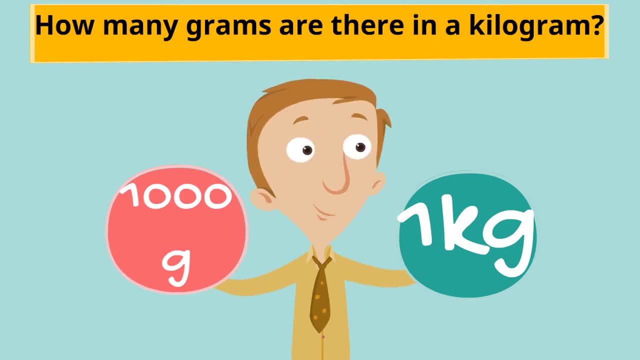 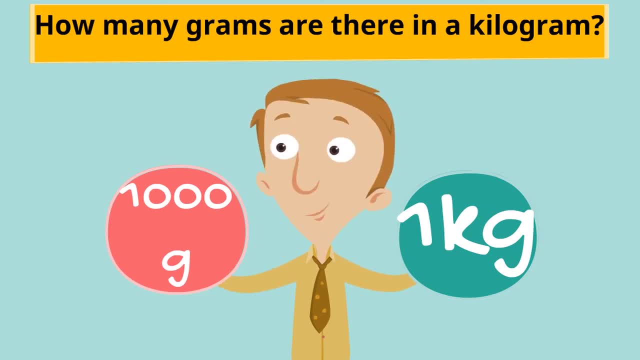 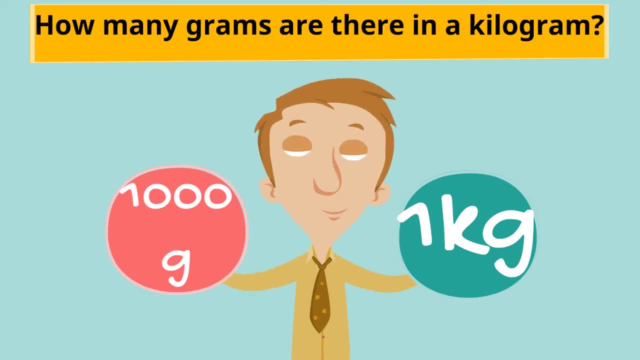 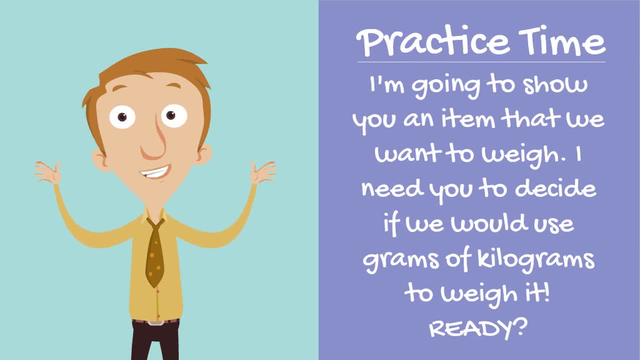 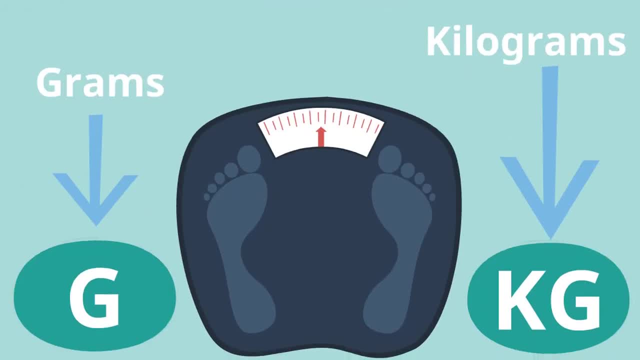 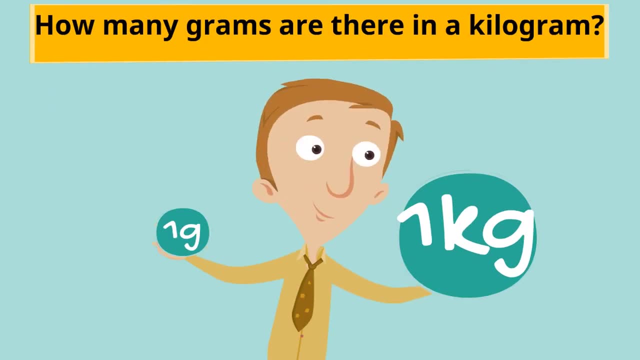 Remember we said we use grams for lighter objects and kilograms for heavier. Well, how many grams do you think there are in one kilogram? If you're very sharp, you might notice that little word kilo before the word gram in our bigger unit. 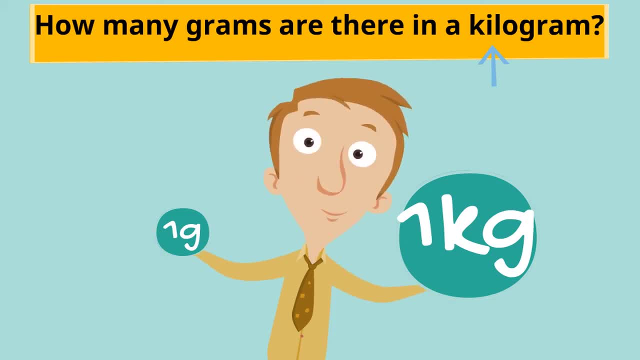 And if you can remember from last week's lessons on length, we saw that word kilo there as well. So if you're very sharp you might notice that little word kilo there as well. So that might help you figure it out. 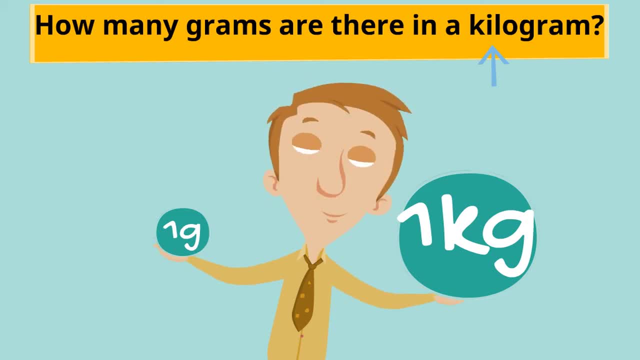 Pause the video and write down how many grams there are in a kilogram. Well, did you get it right? There are 1,000 grams in a kilogram. Remember that word kilo means 1,000 of, just like a kilometre. 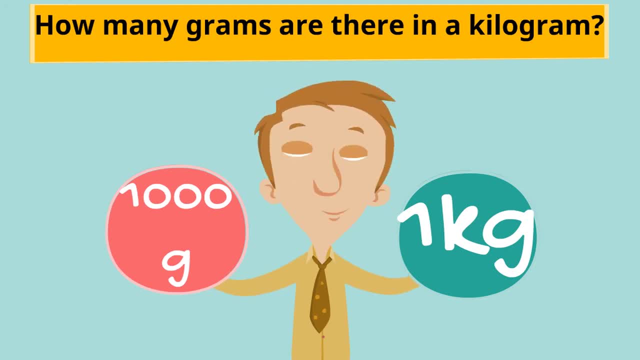 If you want to feel how heavy one kilogram is, maybe check in your presses to see if you have a bag of sugar. These are usually 1 kilogram heavy, So you can feel it in your hand and see roughly how heavy a kilogram is. 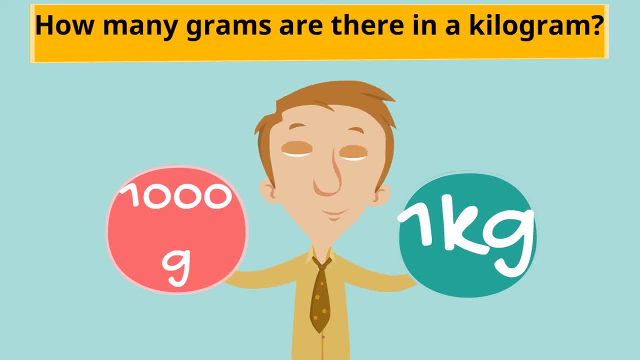 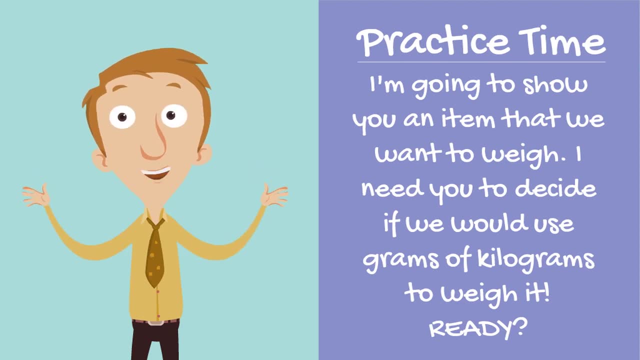 OK, now that we know that there's two different units of measuring weight- one for lighter objects, one for heavier objects- it's time to do a little practice. I'm gonna show you an item that we want to weigh. I need you to decide whether we would use grams or kilograms to weigh it. 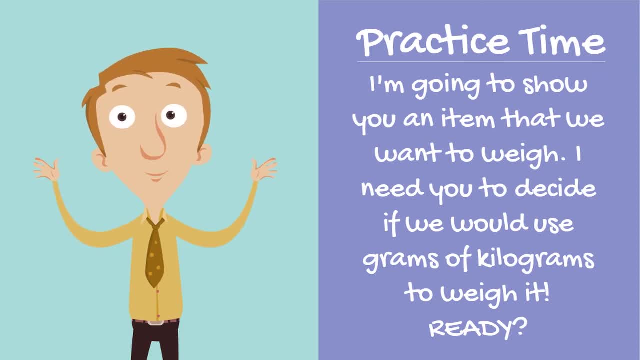 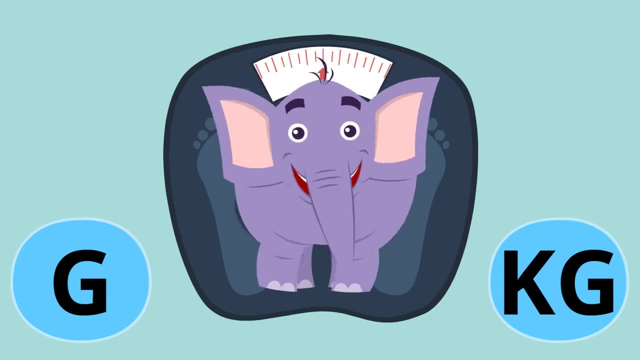 And that's going to be quite a lot of different things. So here it is, Here it is. Come on 7.5 kg. it You ready? Okay, here's your first item we want to weigh. Would we use grams or kilograms? 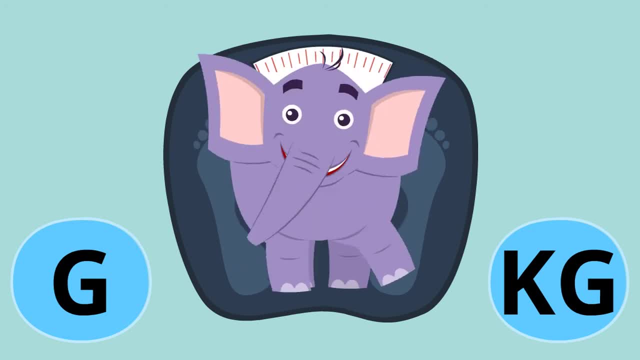 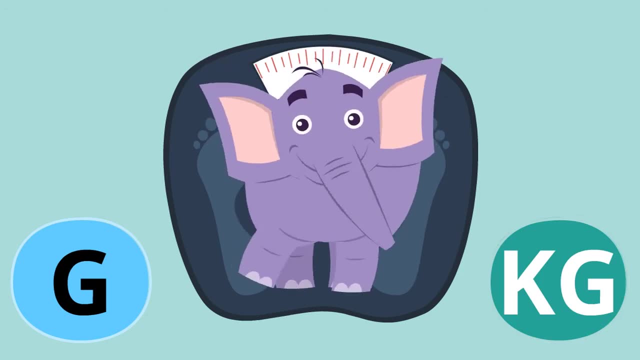 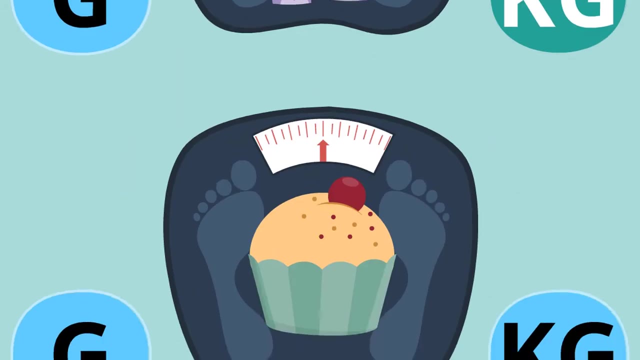 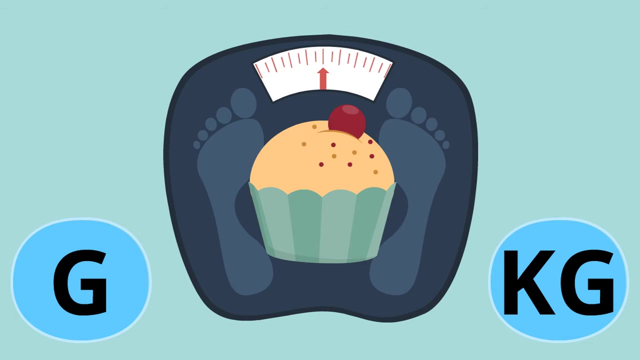 to weigh this elephant. Pause the video and write down your answer. Well, of course, to weigh something as heavy as an elephant, we would use kilograms, the bigger unit of measure. Next one, This cupcake. would we use grams or kilograms to weigh this cupcake? Pause the video. 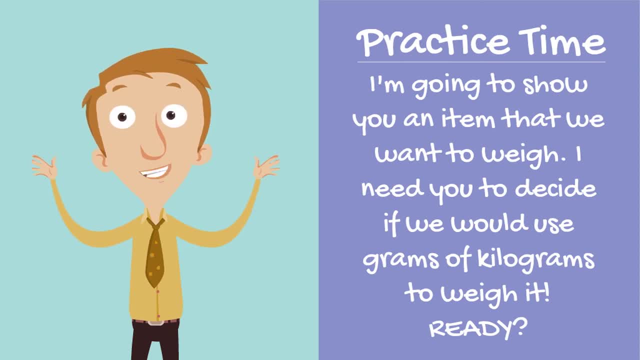 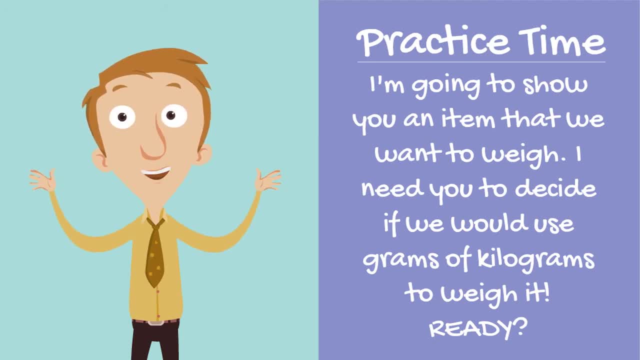 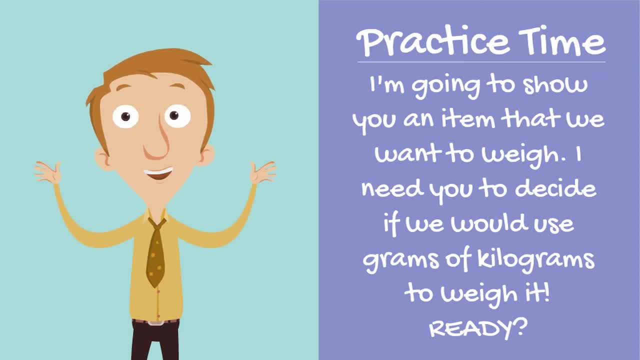 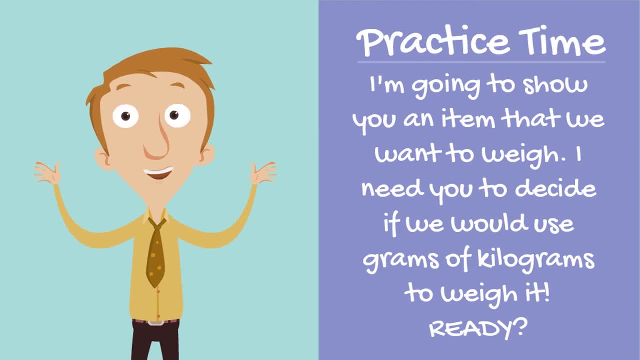 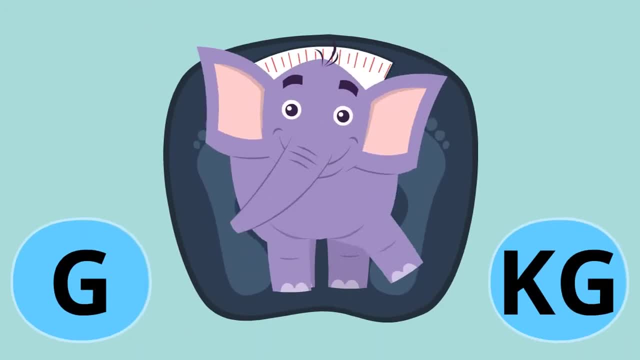 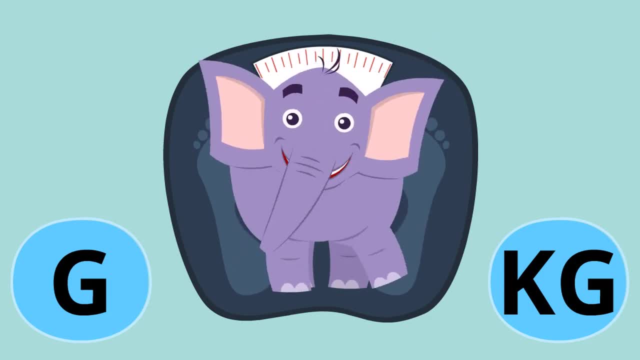 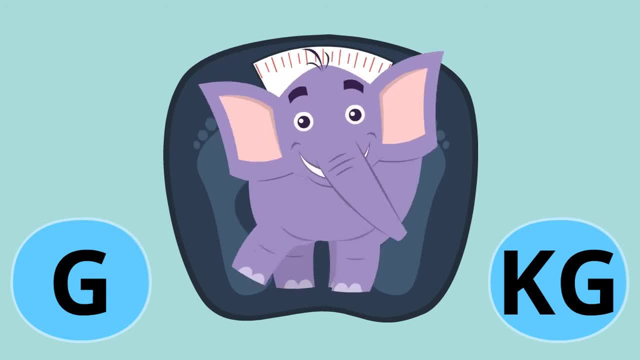 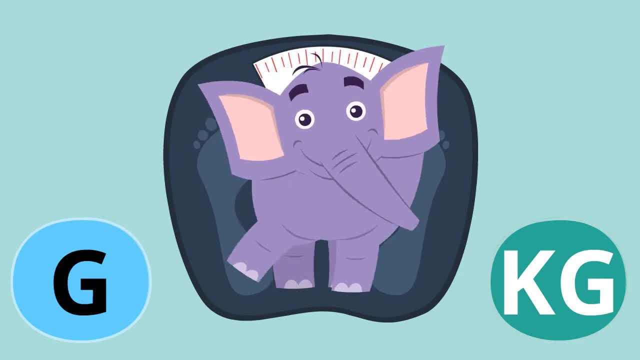 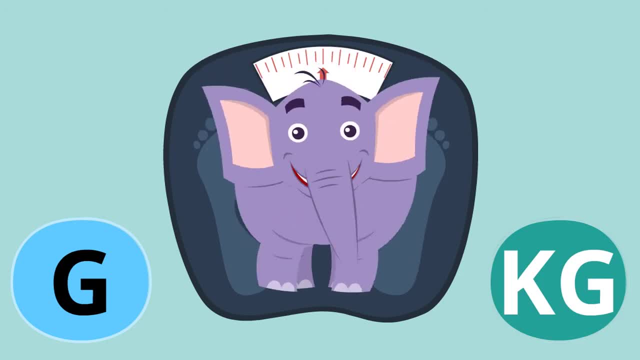 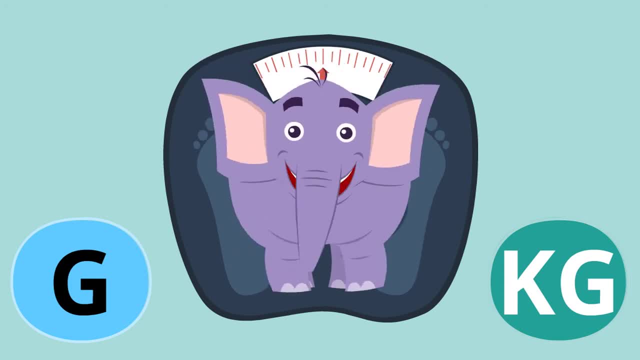 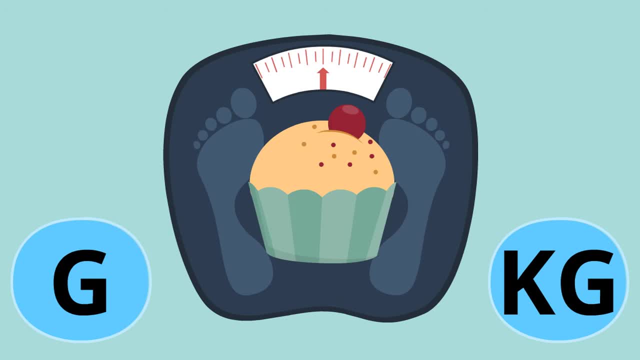 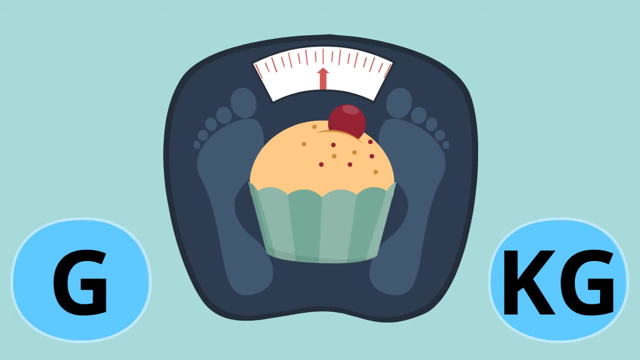 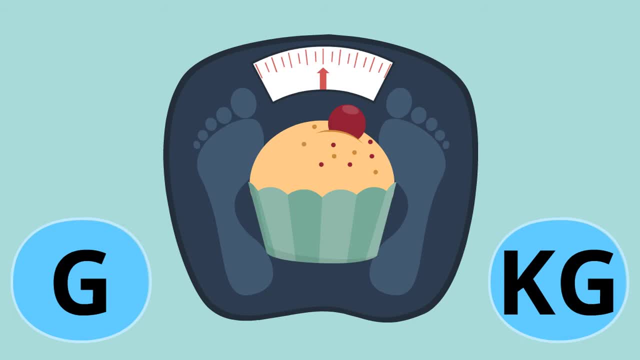 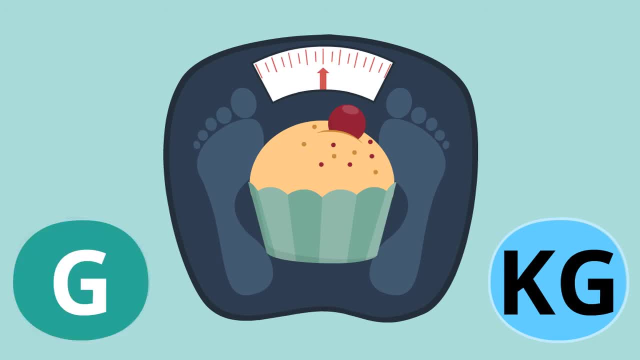 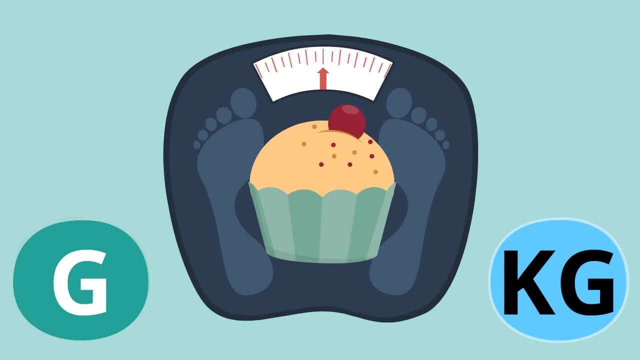 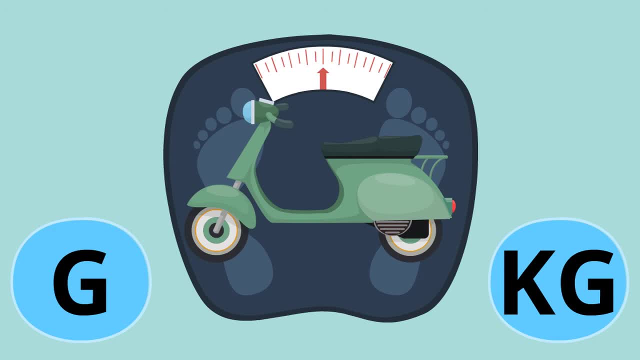 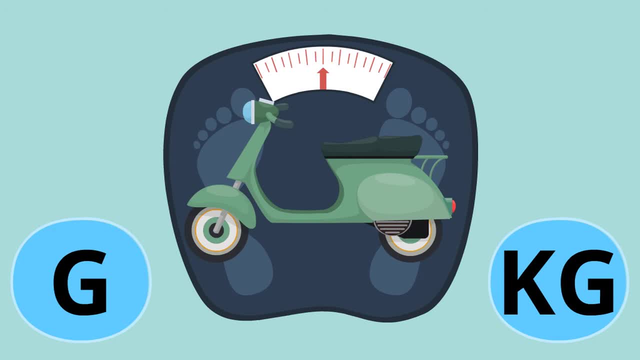 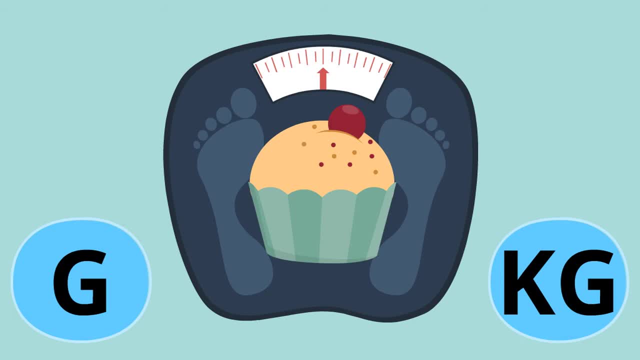 and write down your answer. Well, cupcakes are quite light, so we would use grams to measure this cupcake. Next picture: This moped or scooter. would we use kilograms or grams to weigh this moped? Pause the video and write down your answer. Well, we would definitely use kilograms. 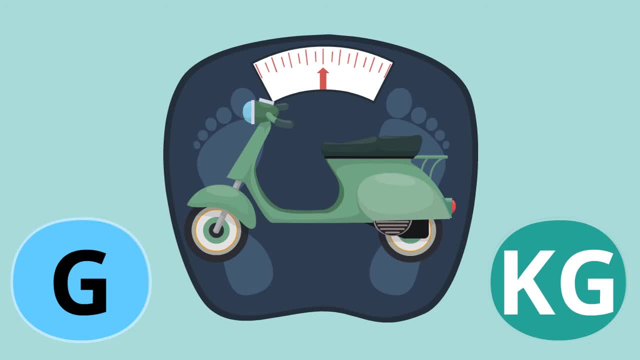 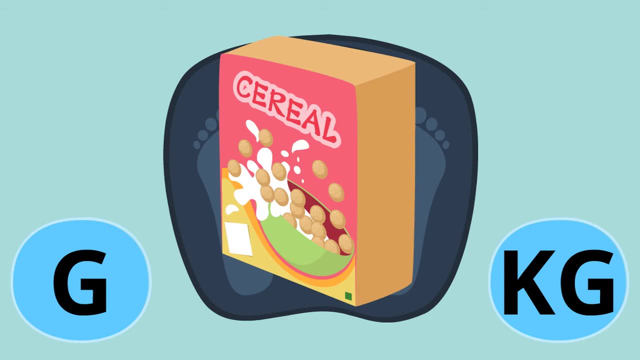 for the scooter, because it's quite heavy. What about this box of cereal? Would we use grams or kilograms to measure a box of cereal? Pause the video and write down your answer. Well, you might have even seen this before. On the side of your box, it usually tells you. 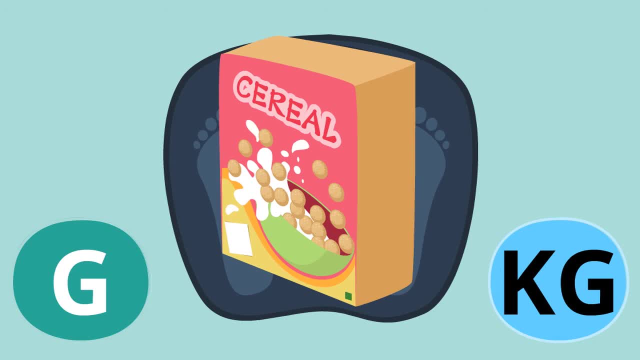 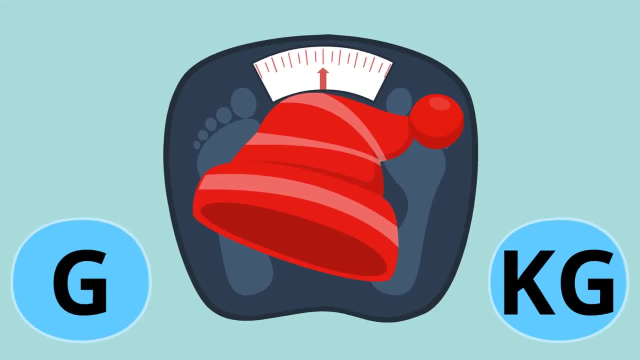 that it weighs 500 grams. so we would use grams to measure the cereal box. And one last one: How about this hat? Do you think we would use grams or kilograms to measure this hat? Well, we would certainly use grams to measure the hat because, again, if it was kilograms, 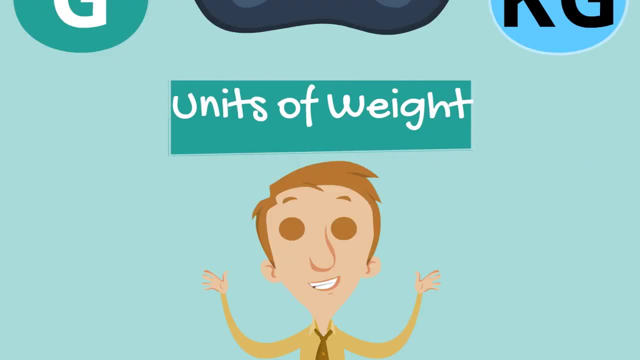 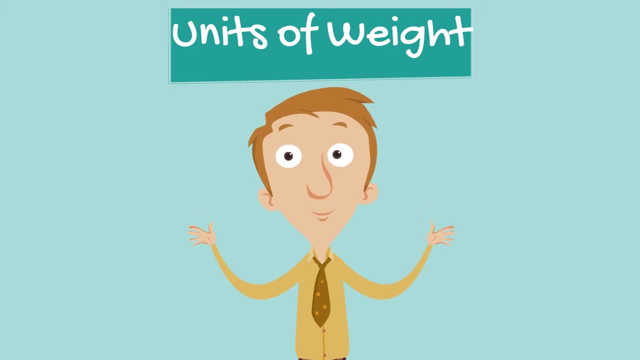 it would squish you down into the ground for being so heavy. It's really useful to have different units of measurement, Such as grams and kilograms, because then we can use them for weighing different objects. And boy do we use them a lot. Weight is used every day in a huge variety of different places. 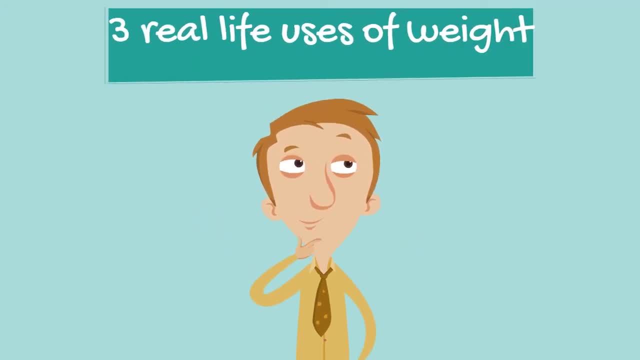 and jobs. Can you think of at least three different places or activities where you would need to be able to use weight? Pause the video and write down your answer. Well, we would definitely use grams. Pause the video and write down those three different answers. 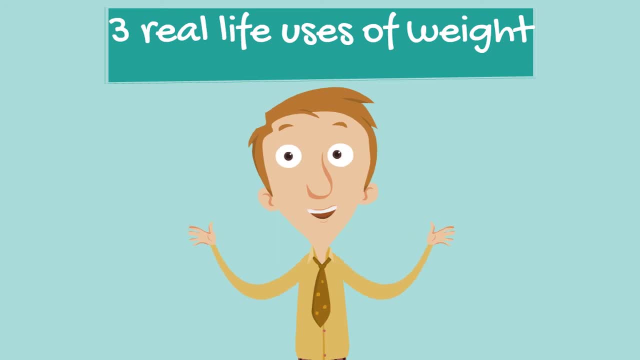 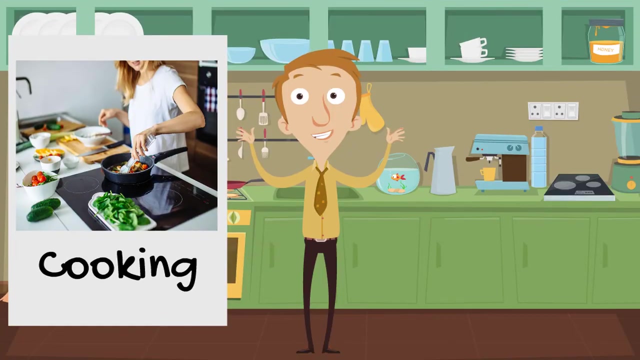 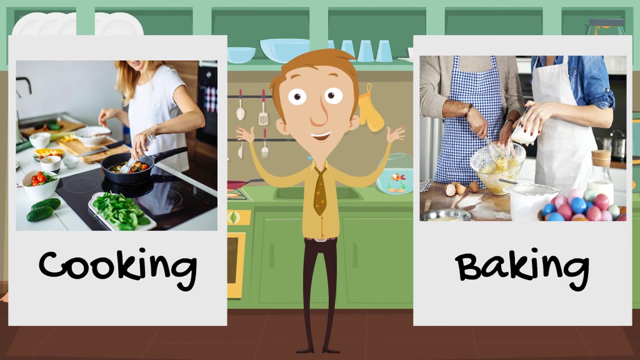 Weight pops up in all kinds of weird and unusual places in the real world. One place where you've probably seen weight before- or if you haven't already, you definitely will once you start doing this- is in the kitchen. Weight is in every single baking recipe, from cookies to fancy wedding. 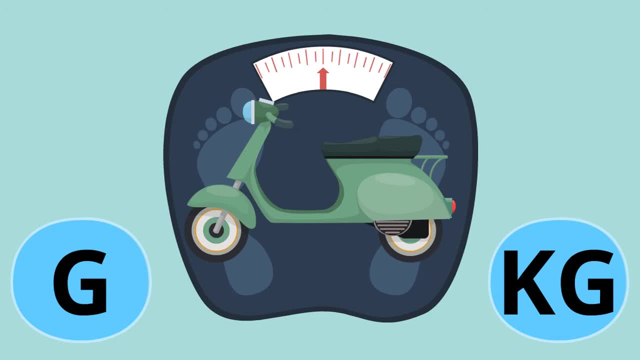 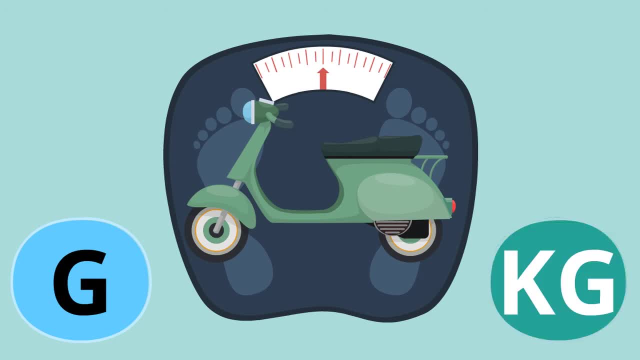 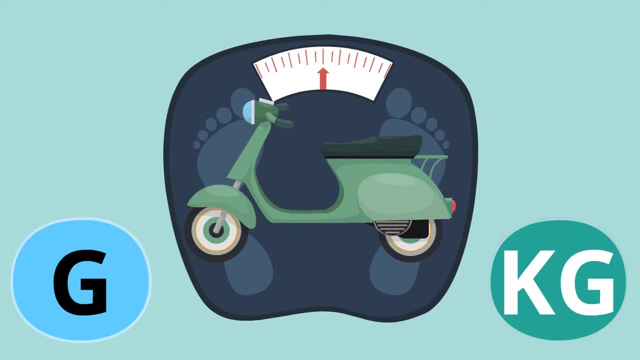 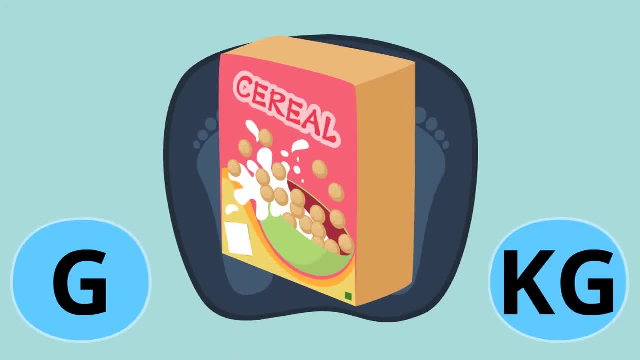 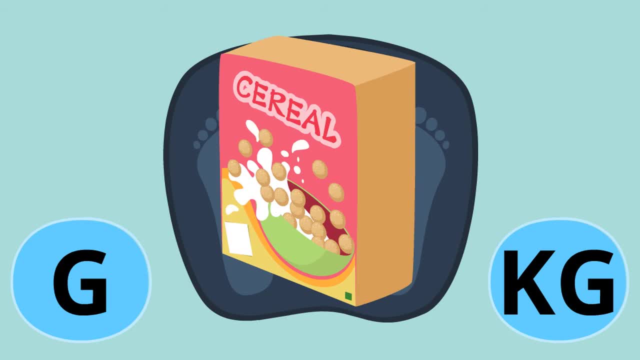 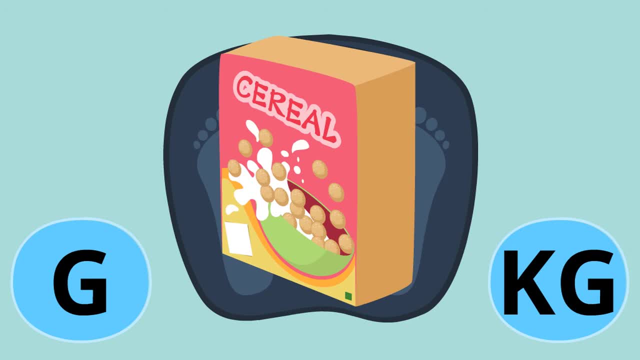 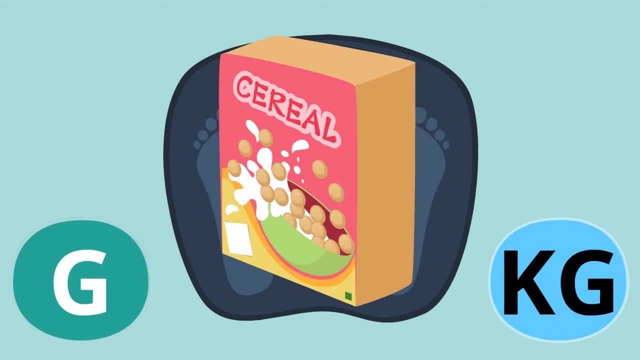 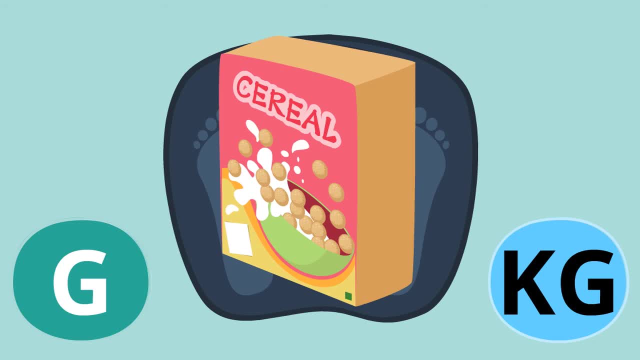 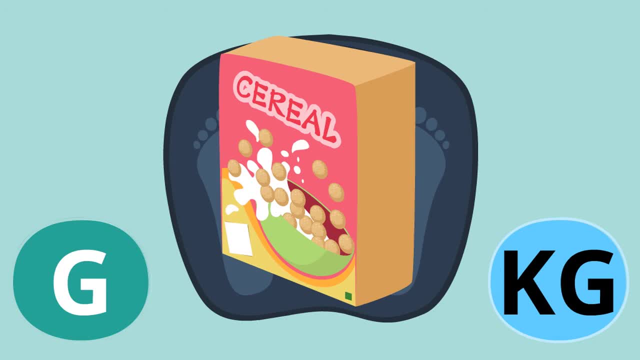 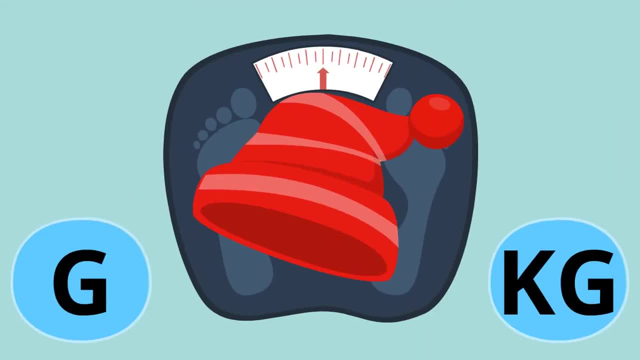 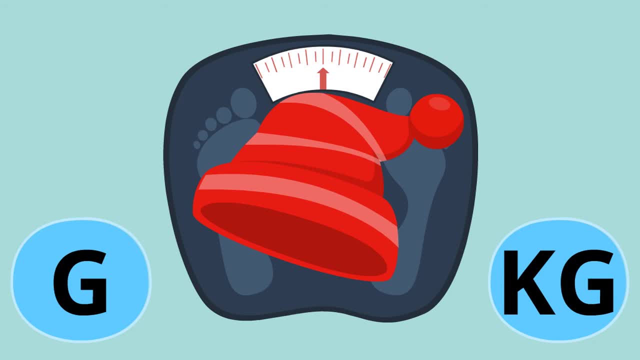 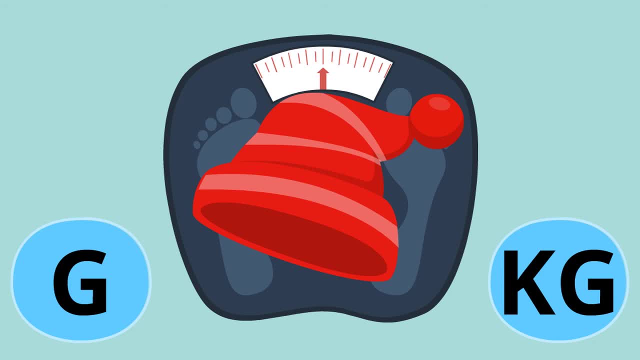 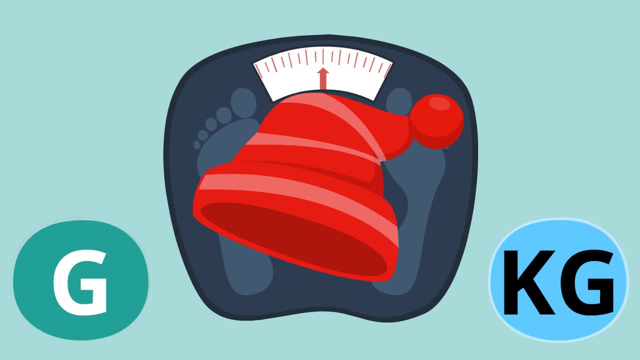 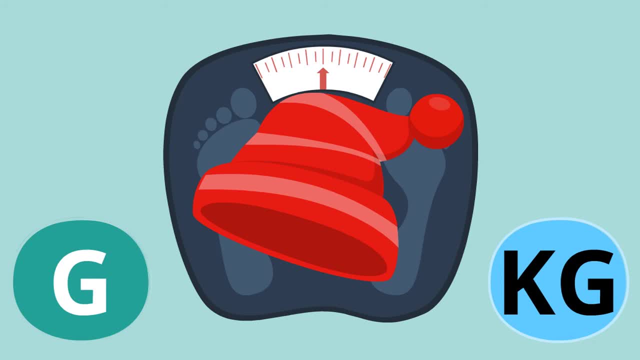 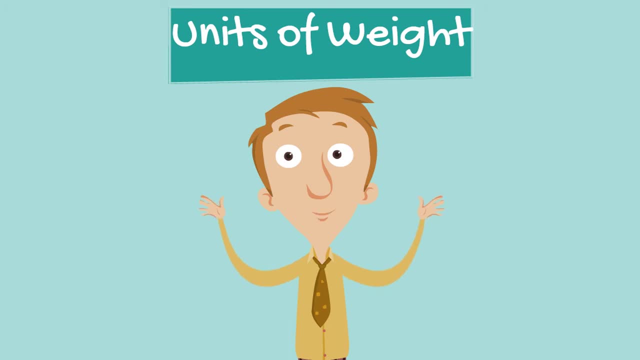 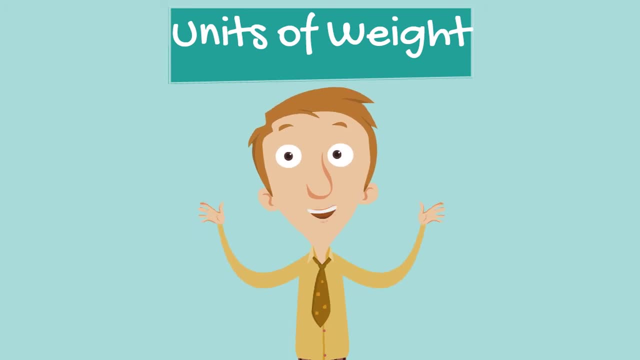 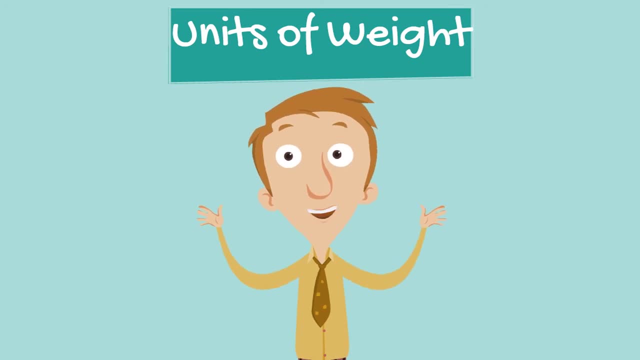 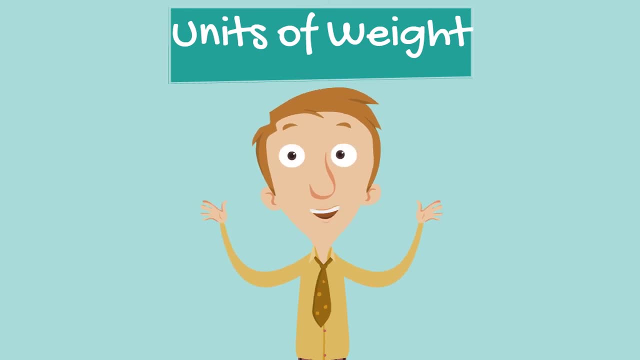 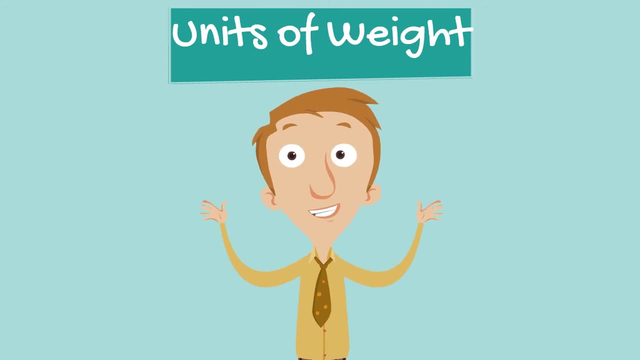 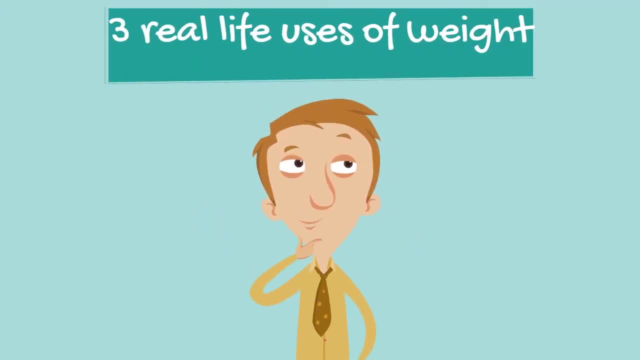 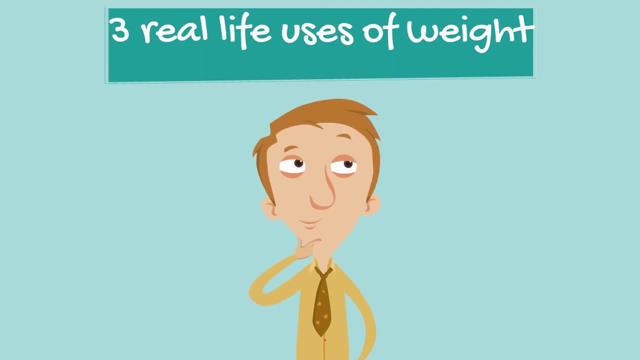 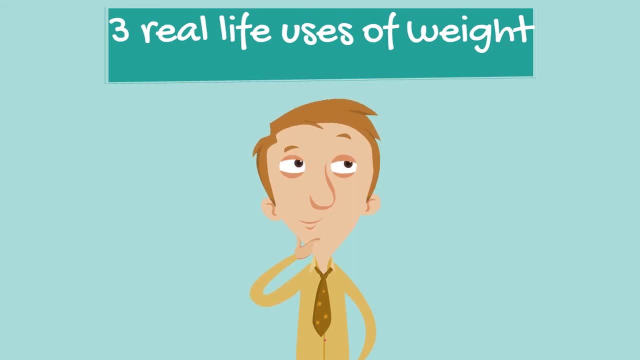 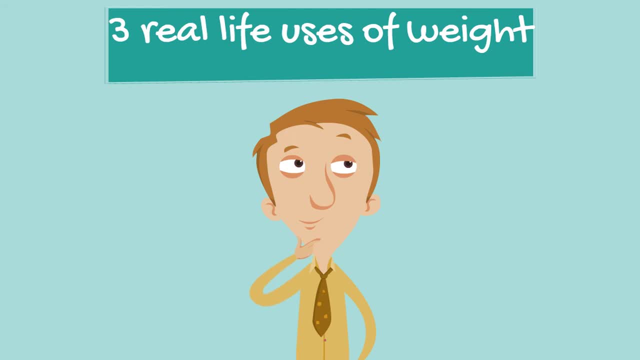 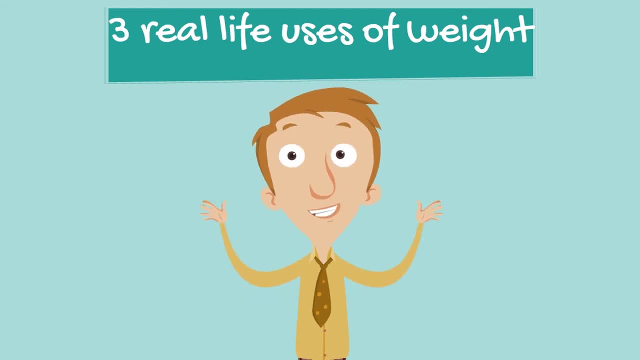 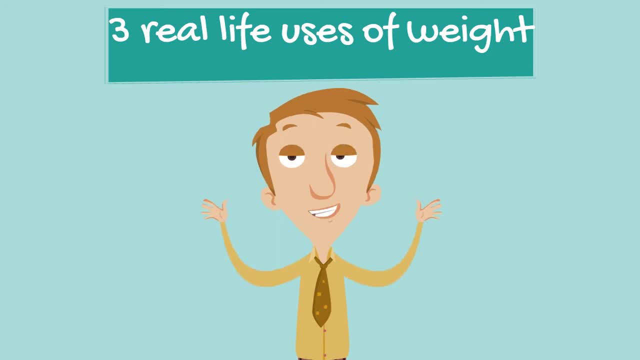 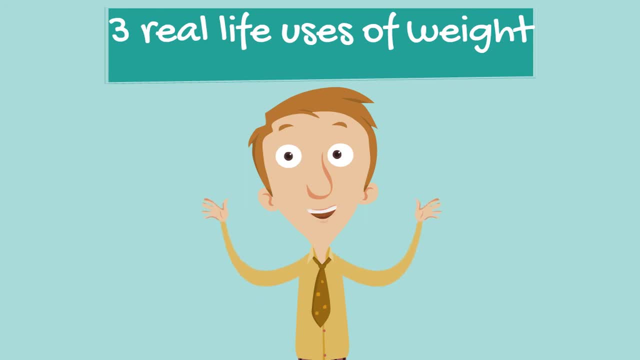 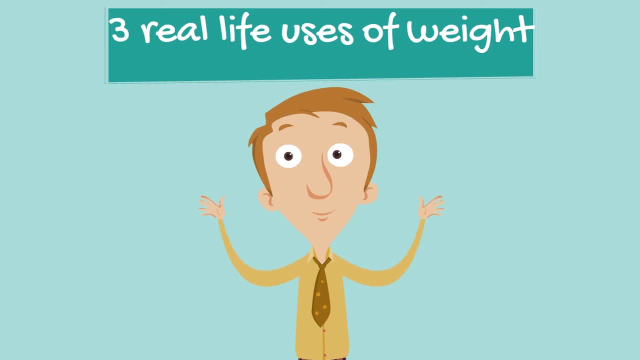 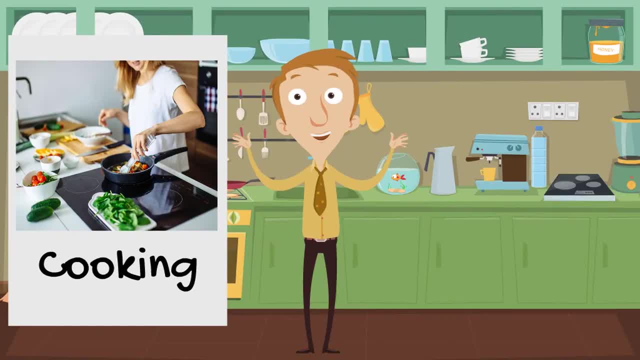 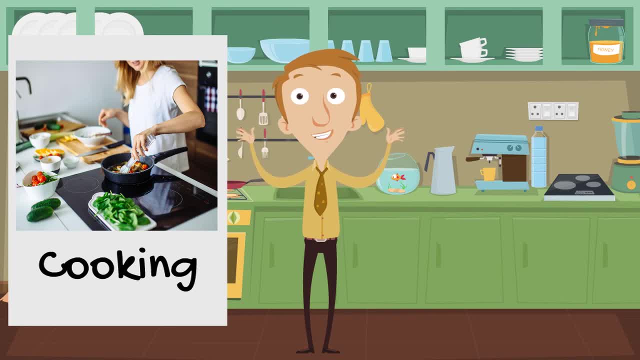 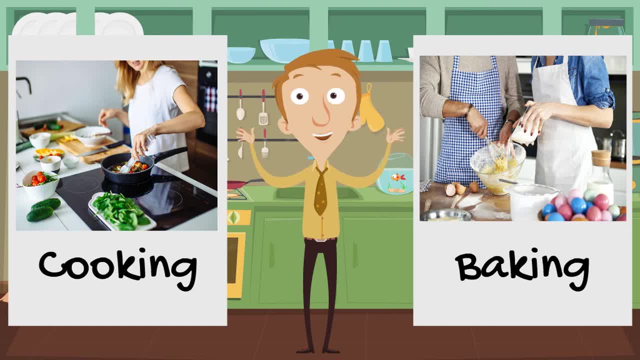 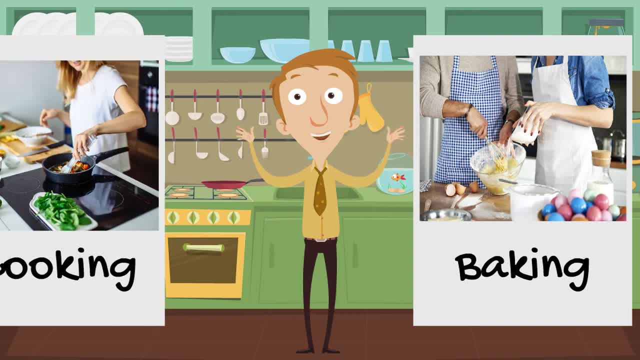 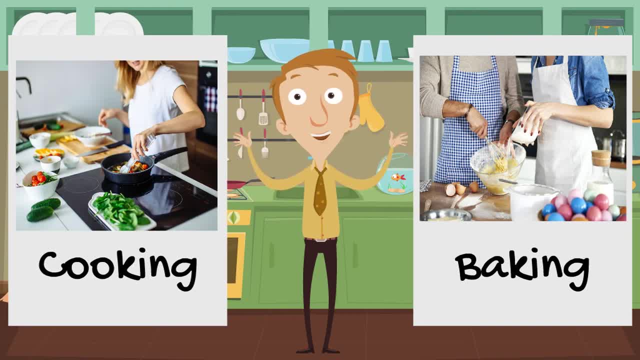 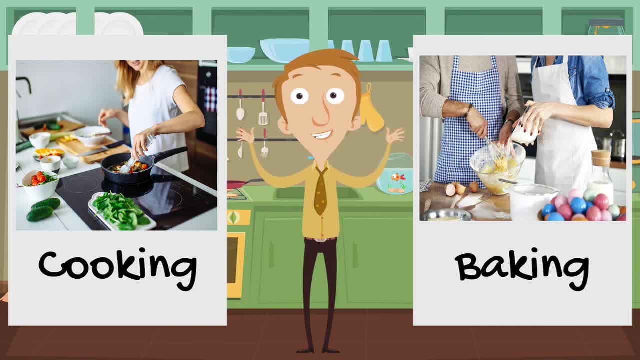 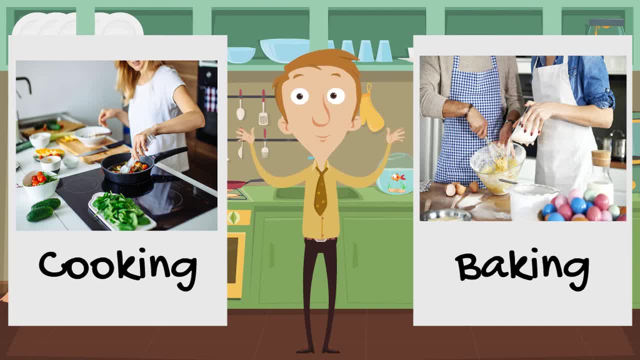 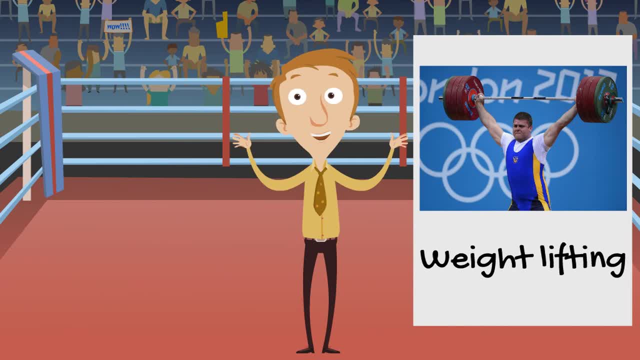 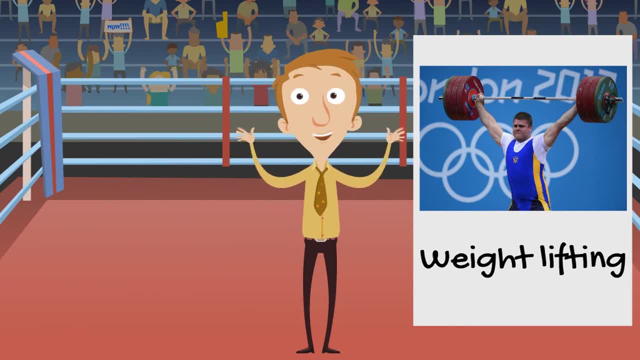 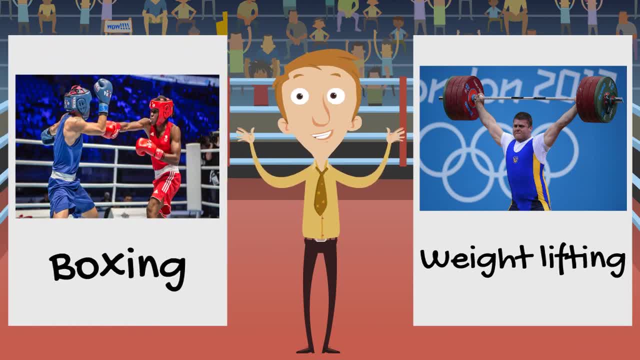 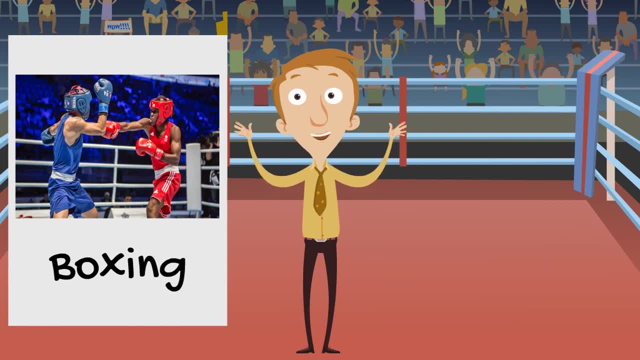 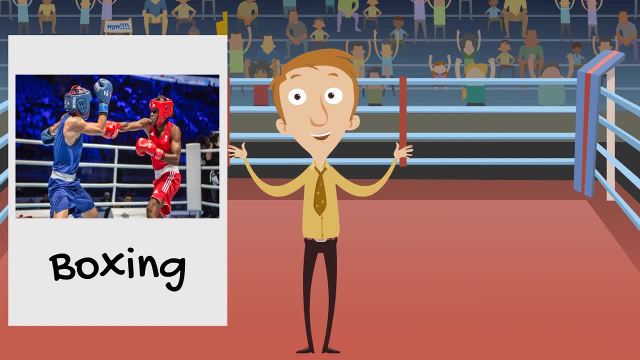 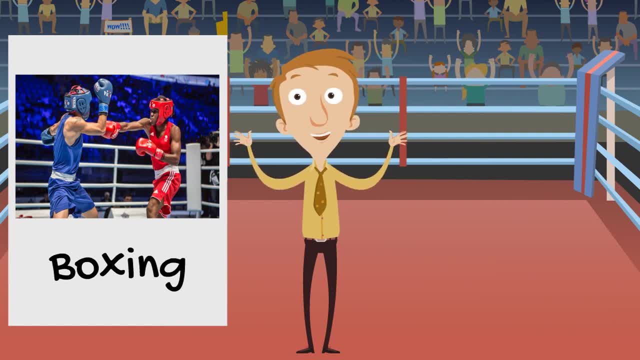 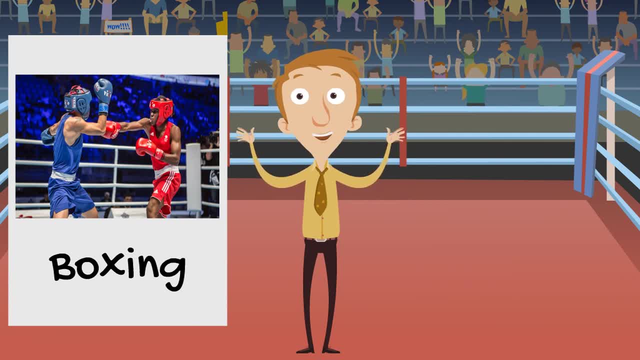 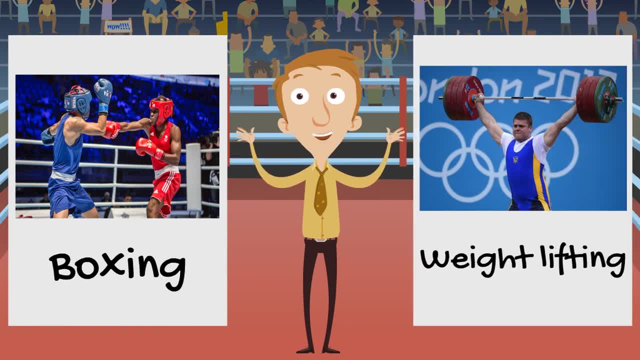 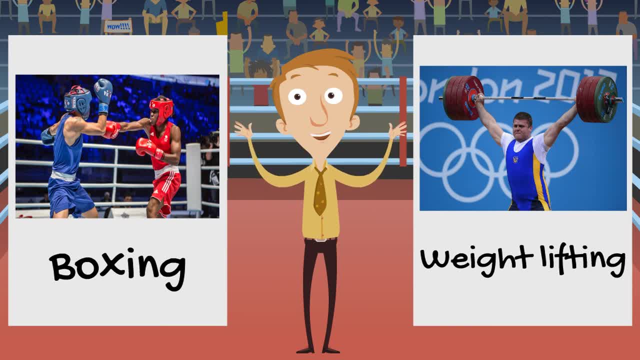 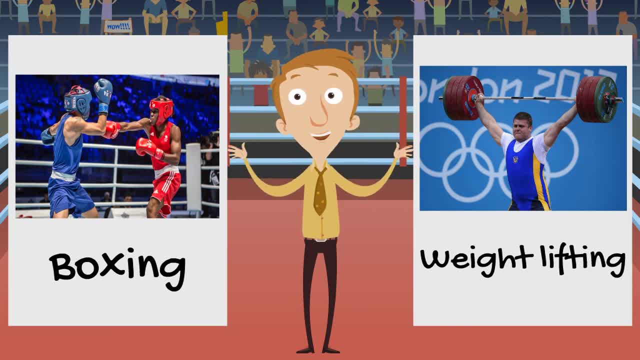 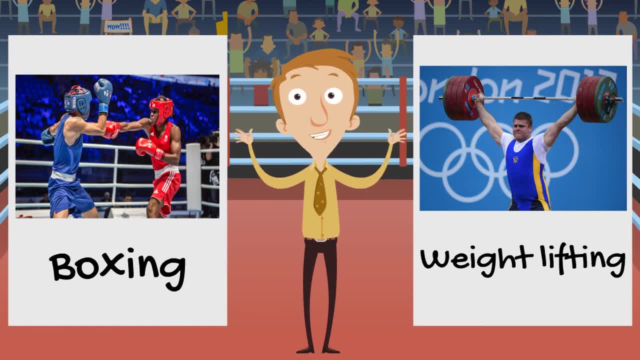 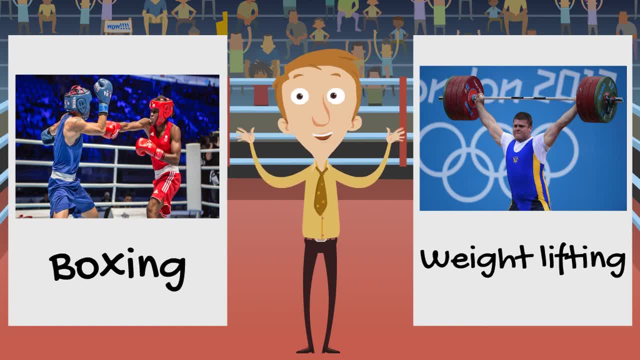 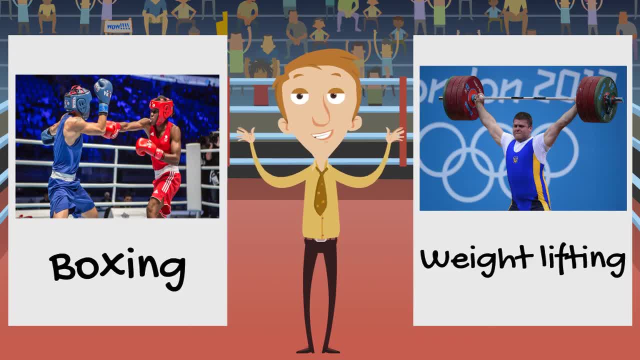 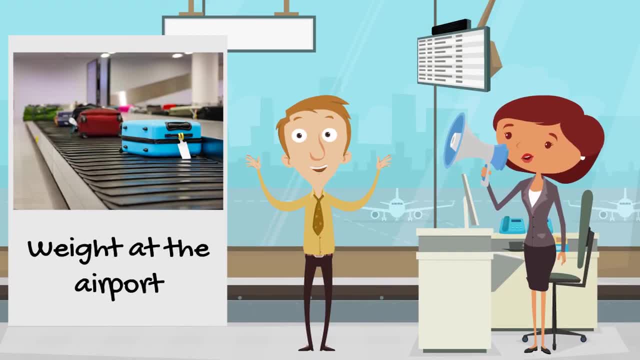 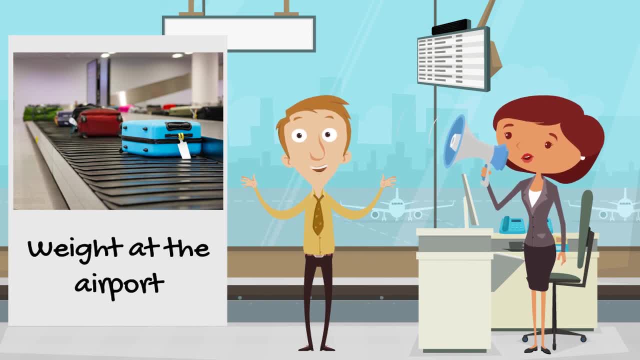 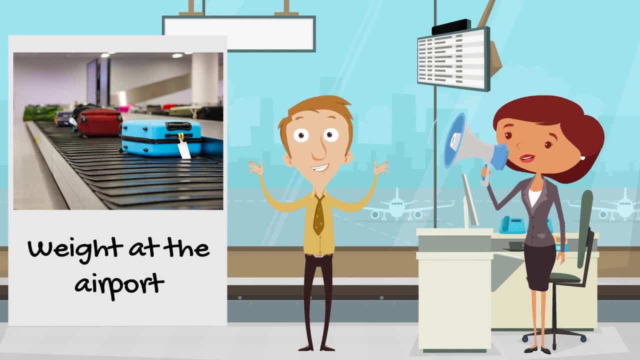 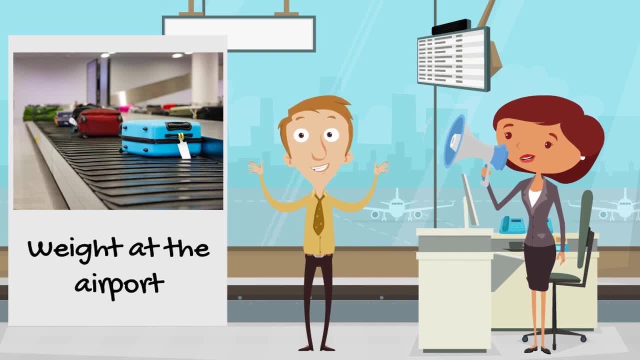 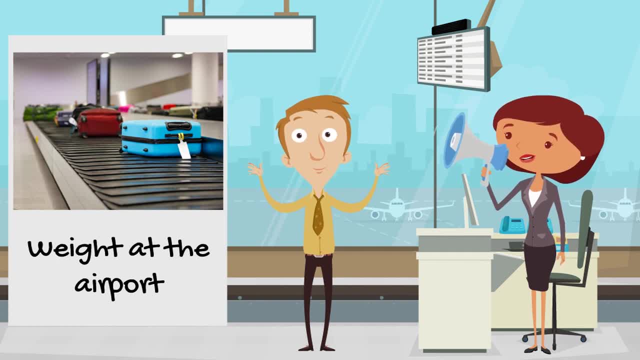 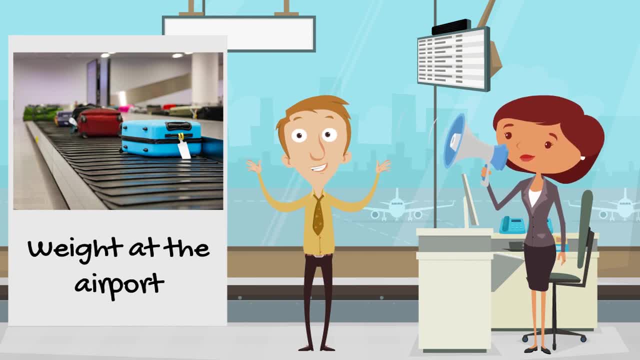 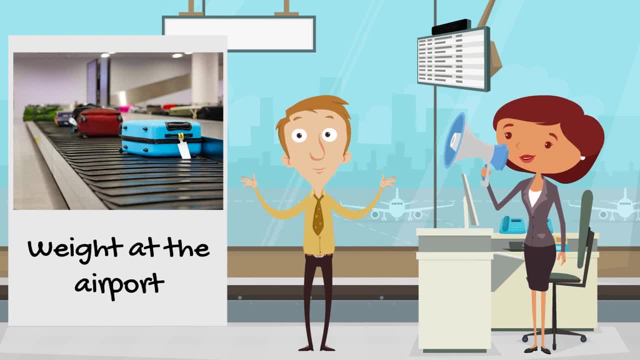 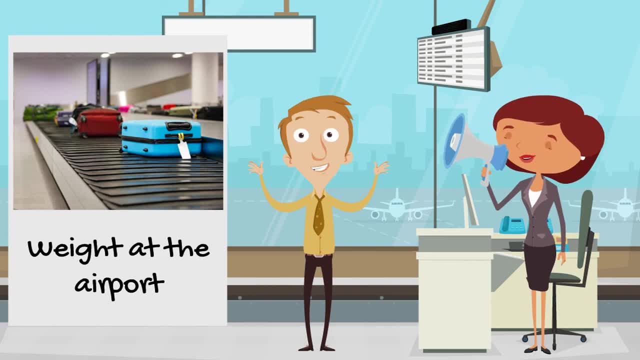 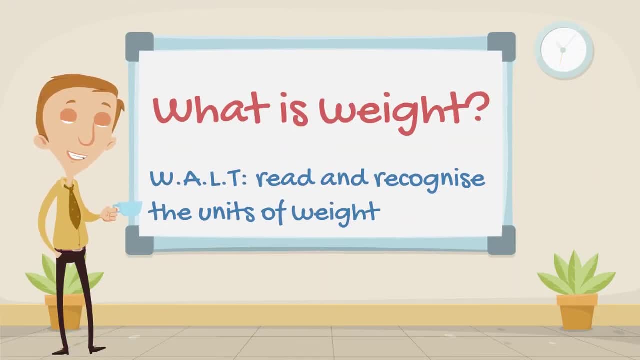 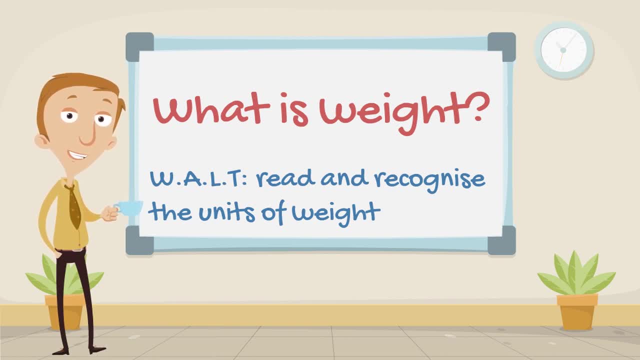 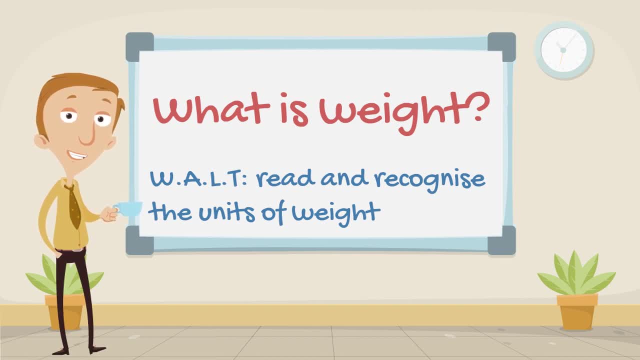 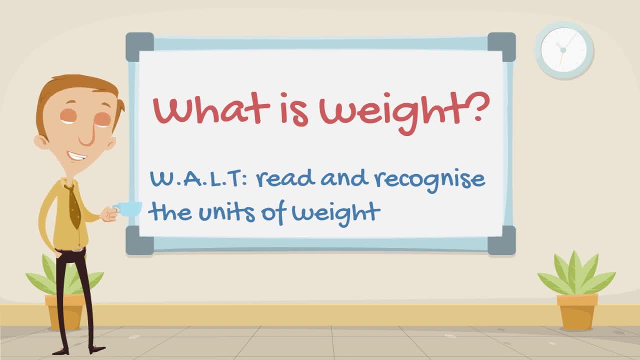 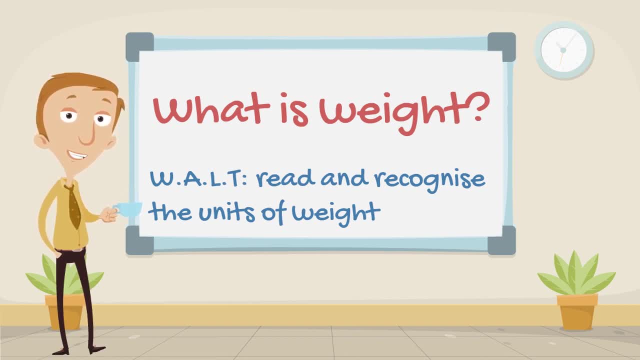 If you want to feel how heavy one kilogram is, maybe check in your presses to see if you have a bag of sugar. 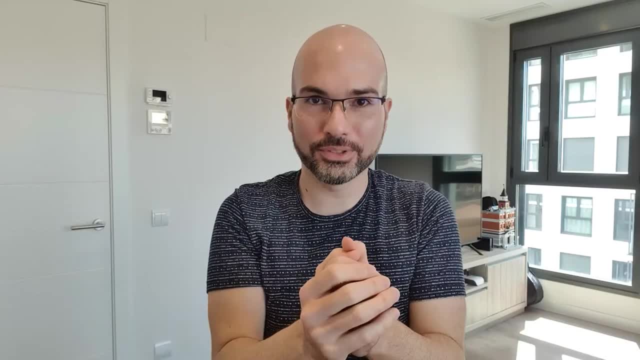 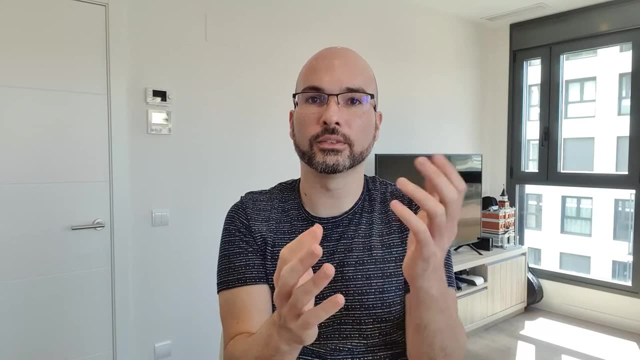 Hello there and welcome to my channel. I'm Cristian and you're watching a dev story. There are several programming techniques and algorithms that allow you to solve a problem in an easier way. A couple of these techniques are recursion and dynamic programming. Let's talk a. 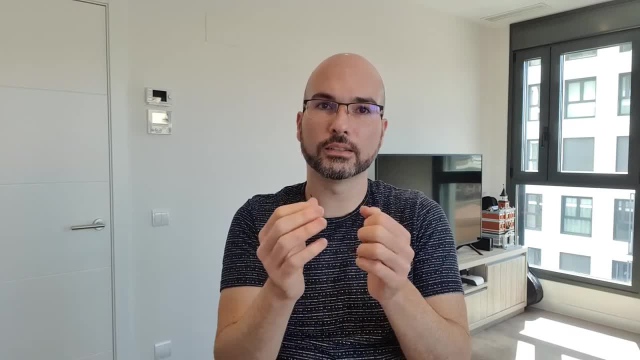 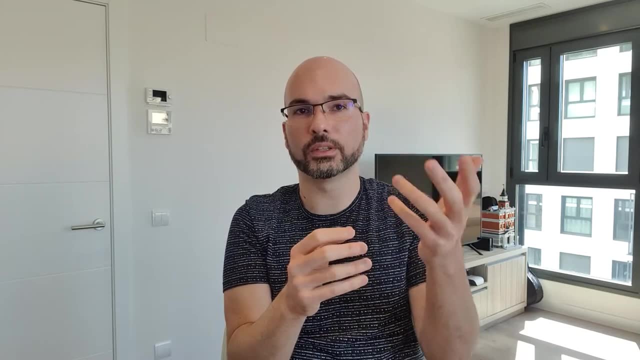 little bit about them. So basically, recursion is a function that is part of the definition right Like? think about factorial or fibonacci, that are the most common recursive function. In factorial number n is the factorial of n multiplied by n minus one factorial and right. 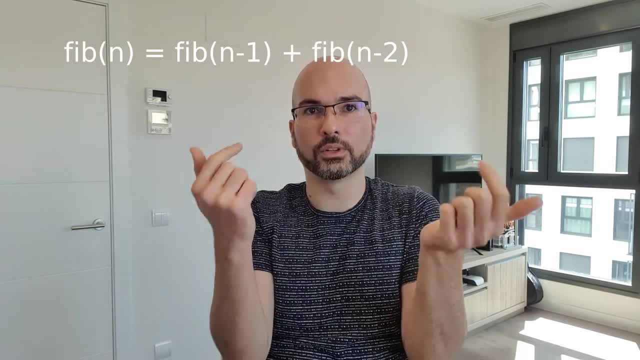 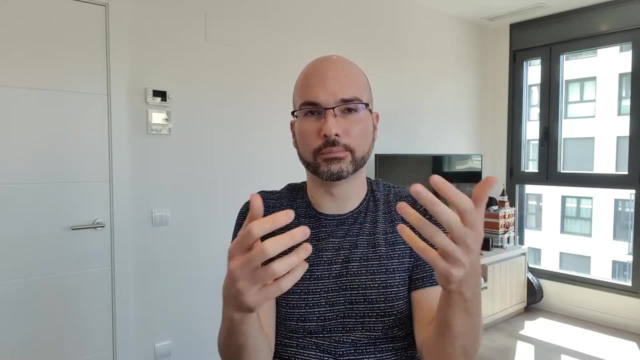 in fibonacci, for example, is a function based on the result of the previous two computations of fibonacci, So it's a program that can call itself, and it's also called a divide and conquer, and many algorithms also use this approach to solve problems. Recursion is a good fit when you have 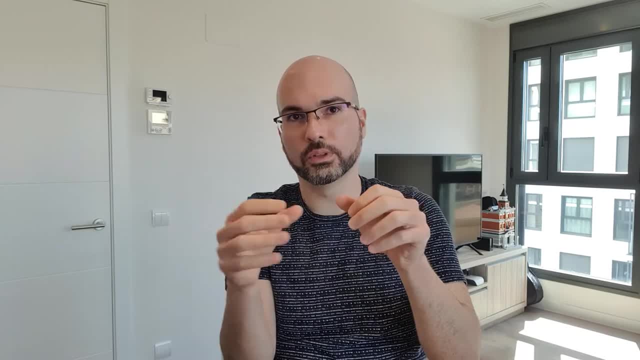 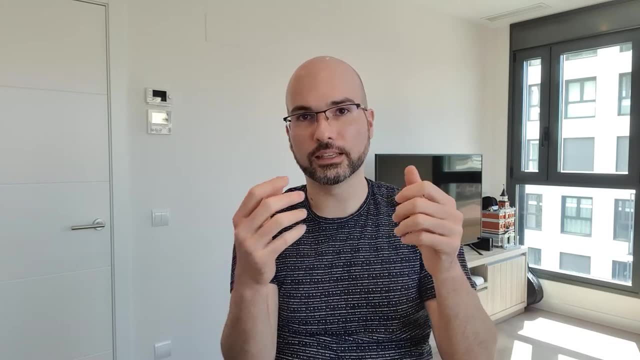 a problem that can be solved by solving two or more smaller problems. Then we have dynamic programming. Basically, dynamic programming is a program that can be solved by solving two or more smaller problems. Then we have dynamic programming. Basically, dynamic programming can be seen as an optimization technique that can be used together with recursion. It's basically